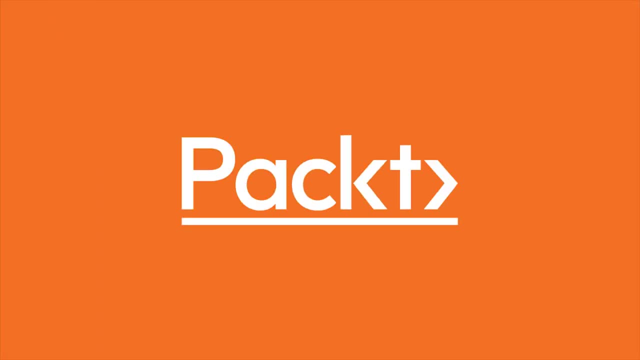 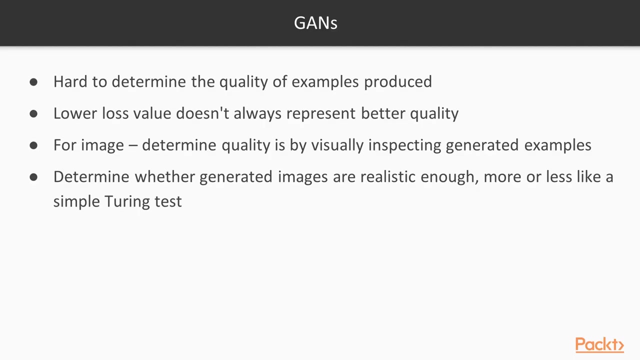 Hello, we're at the new section, GANs and Computer Vision. Let's begin with the first video, Implementing Generative Adversarial Networks. First we understand Generative Adversarial Networks. It is hard to determine the quality of examples produced by GANs. 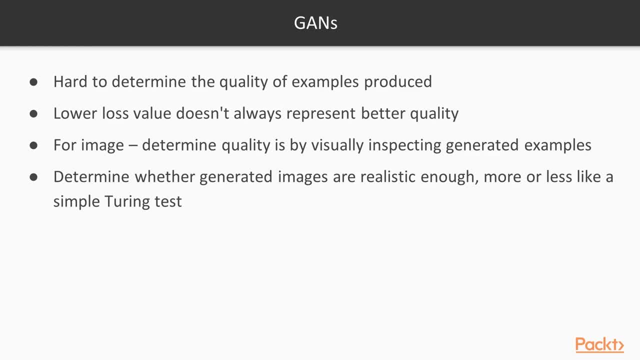 A lower loss value doesn't always represent better quality. Often for images, the only way to determine the quality is by visually inspecting the generated examples. We can then determine whether the generated images are realistic enough, more or less like a simple Turing test. 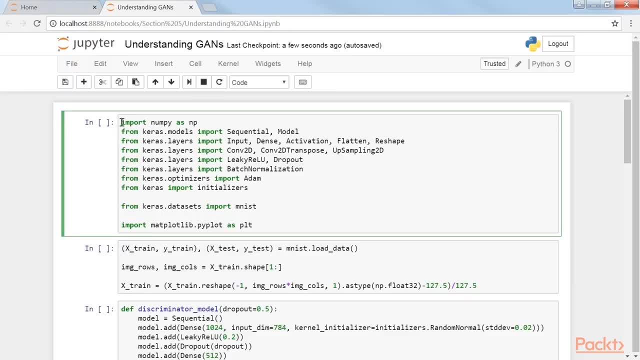 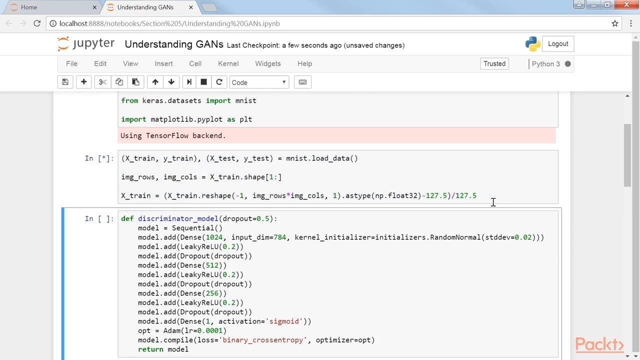 In this video we will introduce GANs by using the well-known MNIST dataset and the Keras framework. We start by importing the necessary libraries. By using Keras, we can easily import both datasets with these lines of code. For our GAN, we need to define three network architectures. 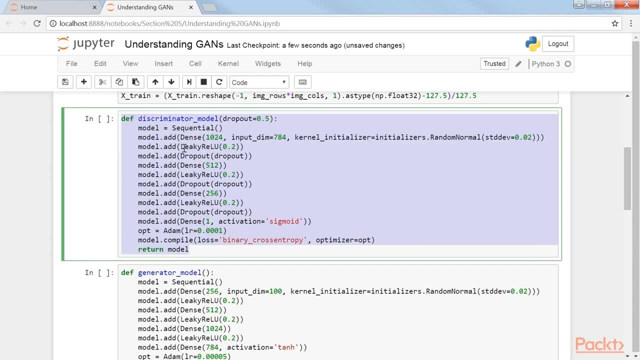 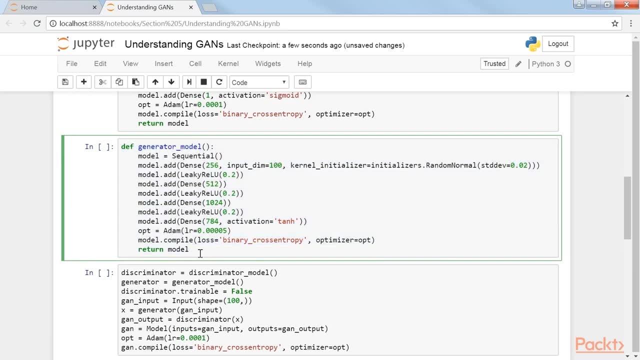 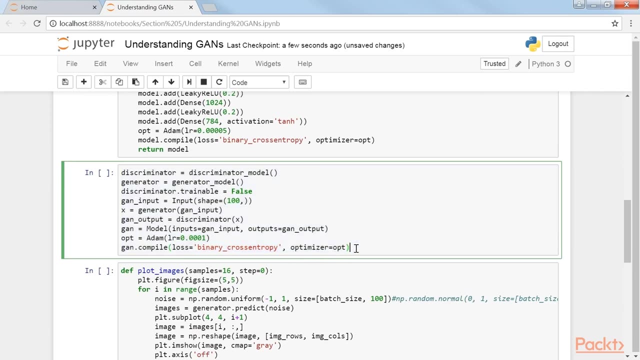 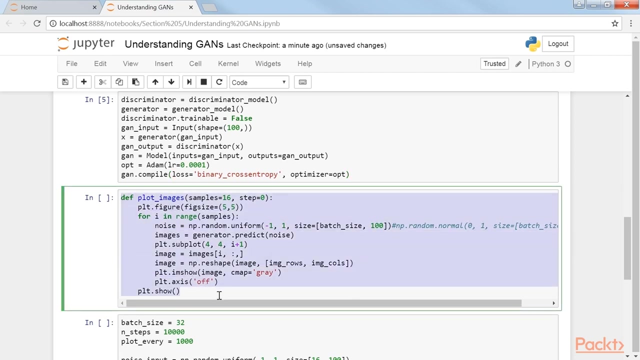 Let's start with Discriminator Model using these lines of code. Next, we will define Generator Model using these lines of code. Finally, we can create our networks and the combined network using these lines of code. Before we train our GAN, we need to define a function to plot the generated images using this code snippet. 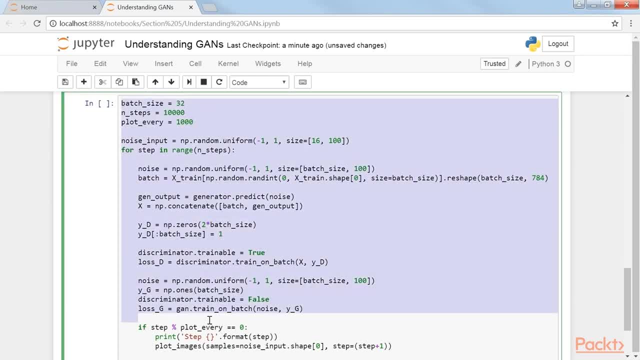 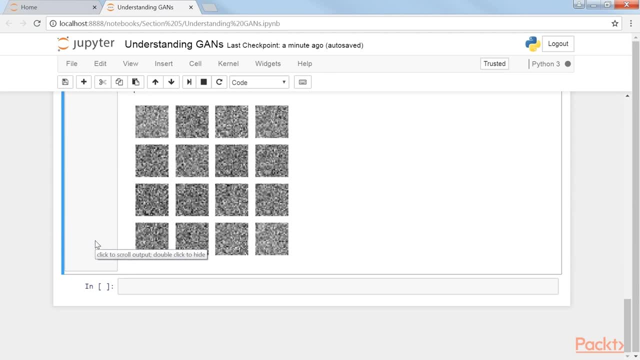 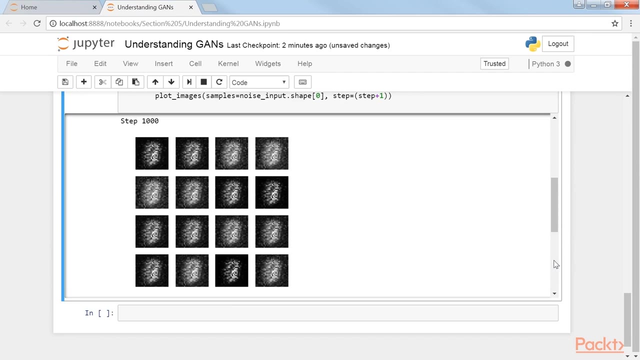 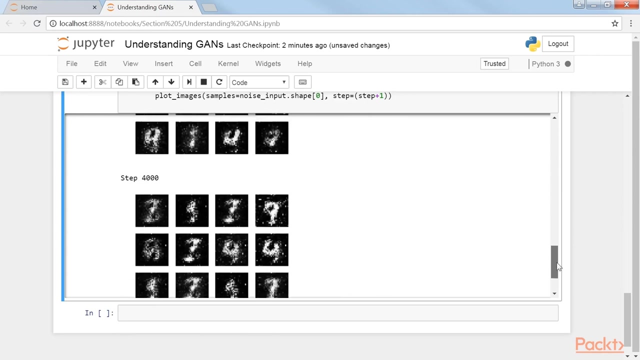 We will now start training our GAN. While training our model, we will output the results. This is the output after 2,000 steps, then 3,000 steps and then 4,000 steps. This is the output that we will get after 5,000 steps. 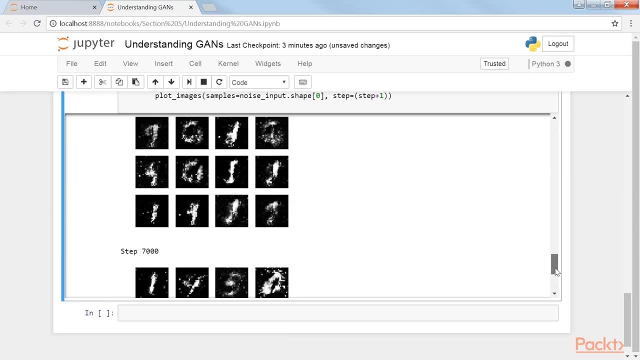 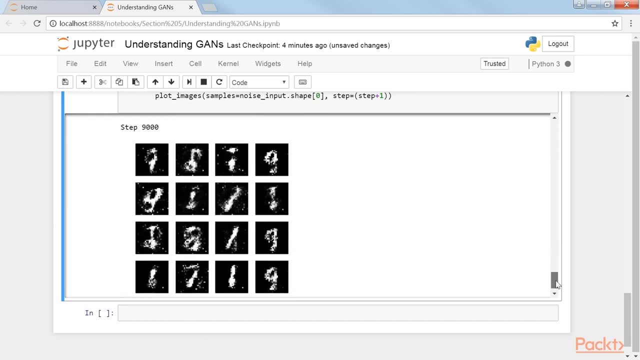 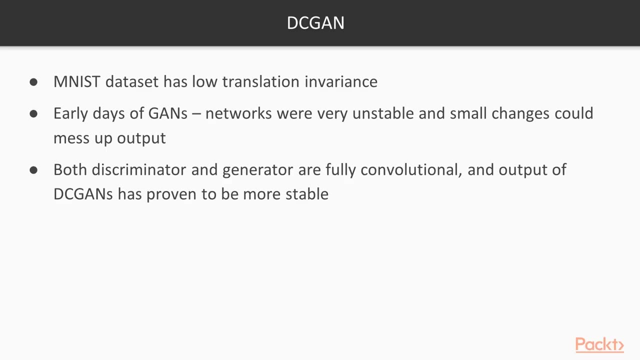 then 6,000 steps, after then 7,000 steps. This is the output after 8,000 steps. Here is the output after 9,000 steps. Now we implement deep convolutional GANs. The MNIST dataset has a low translation invariance.